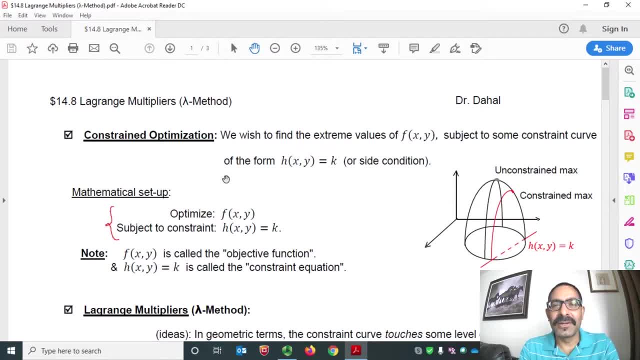 One is constrained optimizations and another one is unconstrained optimizations, And we covered unconstrained optimization in previous section, 14.7.. So today we are covering the constrained optimizations. In constrained optimizations we used to find the extreme values of functions subject to some constrained curve, given of the form h, x, y equals. 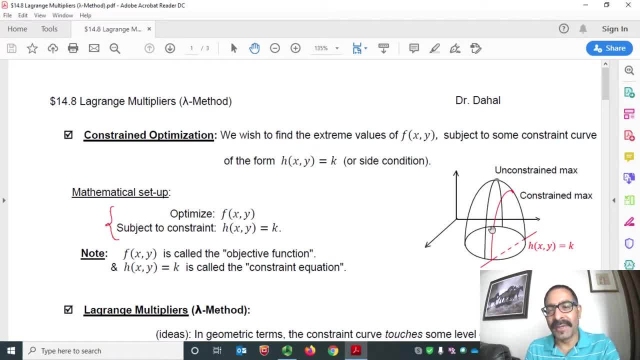 to k. So, for example, in the diagram here we have the upside-down paraboloid. The maximum lies here, which is unconstrained maximum. But if we restrict the domain, or x, y coming from this curve, then its maximum lies here, So the unconstrained. 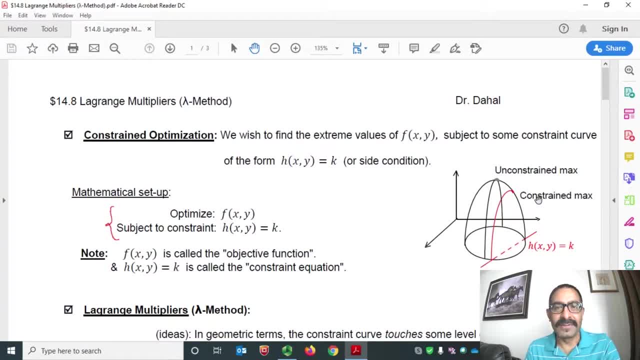 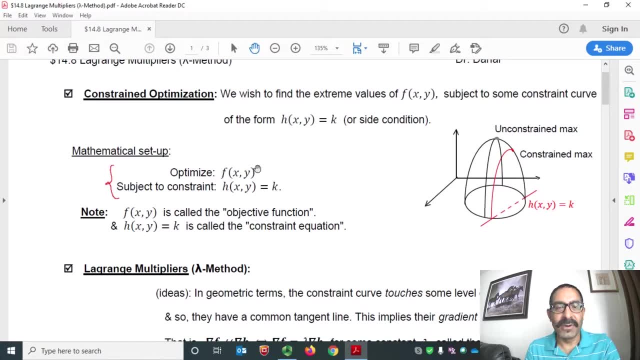 maximum and constrained maximum are different values, So the mathematical setup: we want to use the function f of x y subject to constraint. where x y satisfies this equation, h equals to k. Sometimes the f is also called objective functions and h equals to k is called constrained equations. 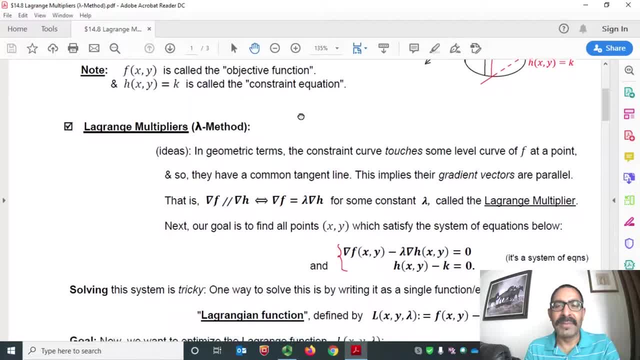 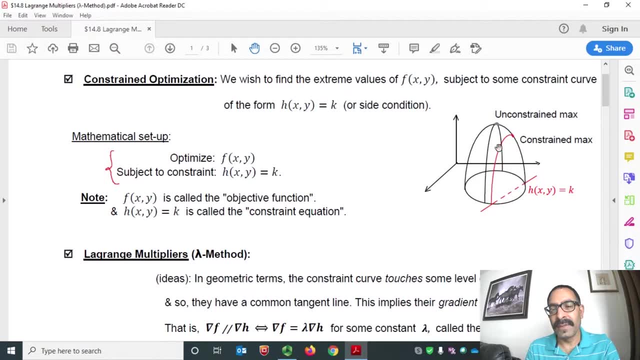 So let's talk about Lagrange multipliers or the lambda method, the ideas In geometric terms. let me go back again to this diagram. So this constrained curve touches some level curves of this surface And at that point of tangency, the tangent vectors at 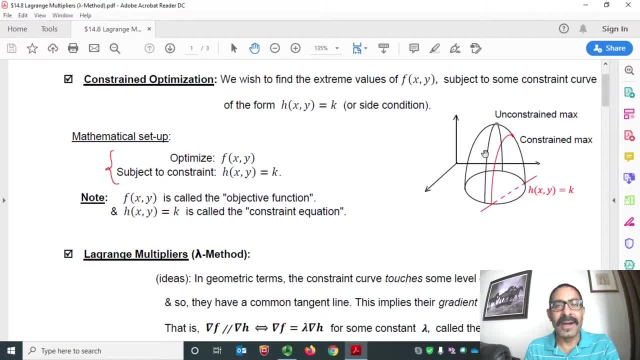 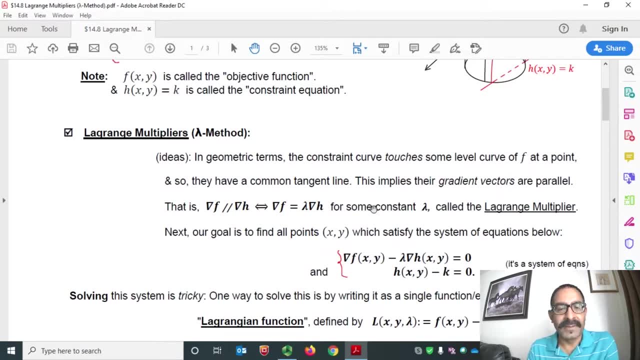 constrained curve and at level curves are the same. So in geometric terms the constrained curve touches some level curves of f at a point, So they have a common tangent line. This implies their gradient vectors are parallel. We know that 2 vectors are parallel if, and only if, one vector is equal to constant. 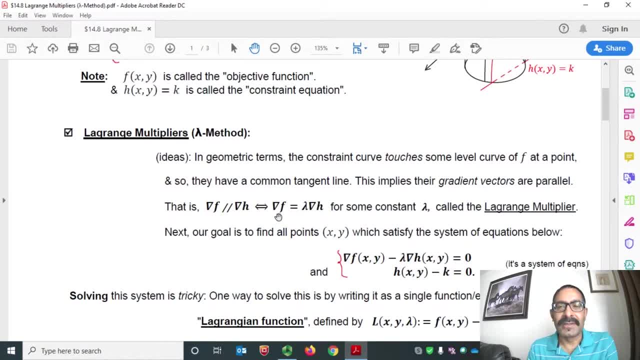 times the other vector. So here gradient f is parallel to gradient h. implies gradient f equals to some constant times the gradient s. We pick that constant as a lambda and that lambda is called the lagrange multiplier. Next our goal is to find all points x, y, which 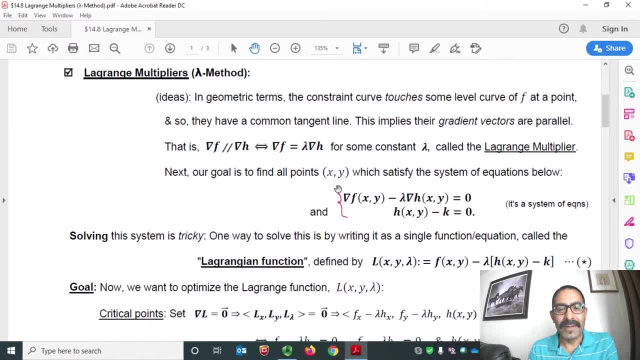 satisfy the system following equations. So here, gradient f minus lambda times gradient h equals to 0 and the constraint here, h minus k, equals to 0. It's a system. Now we want to solve the systems. Solving this system is sometimes tricky. One way is by writing it as a single. 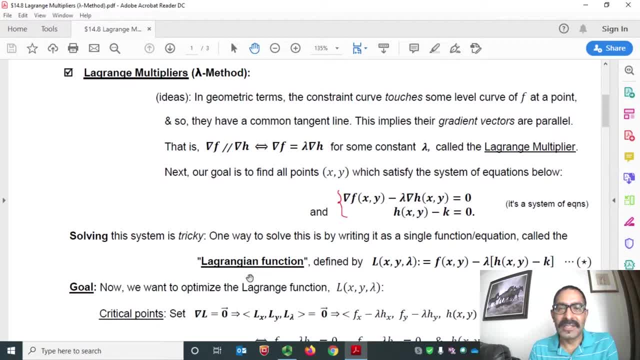 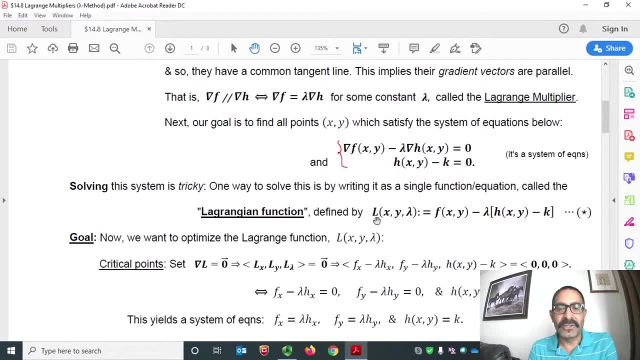 function or equations called the Lagrangian functions, defined by L, x, y, lambda. So L is for Lagrangian x, y lambda equals to the objective functions f, x, y minus lambda times. the constraint f, x, y minus lambda times h, x, y minus k. Sometimes people make mistake here. They sometimes write. 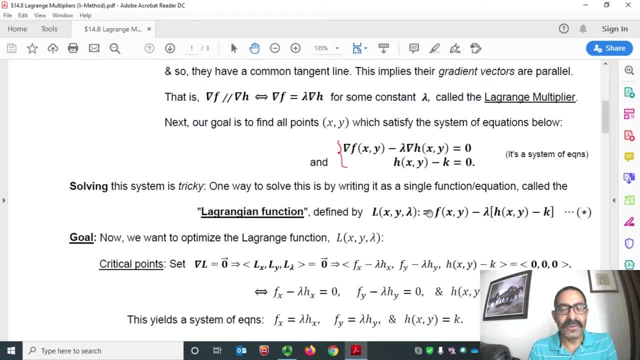 the constraint and then minus lambda times the objective functions. but that doesn't work. So always, we define the Lagrangian function in this way: Objective functions minus lambda times the constraint. here I hope this makes sense to you all. So now our goal is to apply. 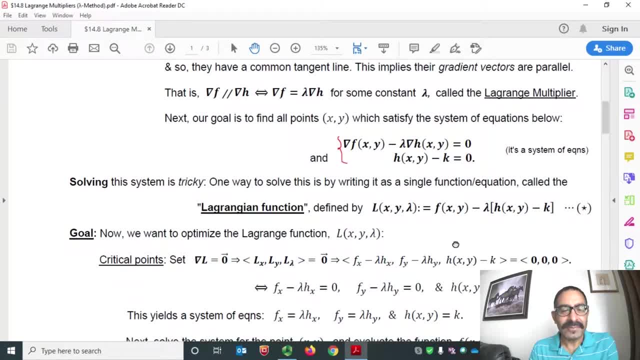 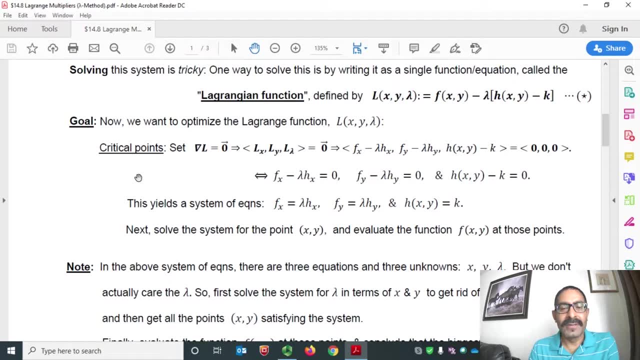 the Lagrangian functions And our idea: first find the critical points. To find the critical point, find the partial derivative of L with respect to x, with respect to y, with respect to lambda. set equals to 0. Find the value of x, y and lambda. But in this method we 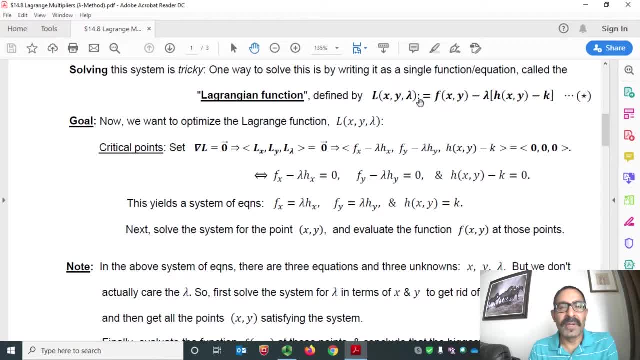 don't care- the value of lambda. Then using the lambda's value we find the value of x and y And we evaluate the function at x and y. So the first: find the critical point. So find the partial derivatives and of L functions and set equals to 0. Then this gives us this: 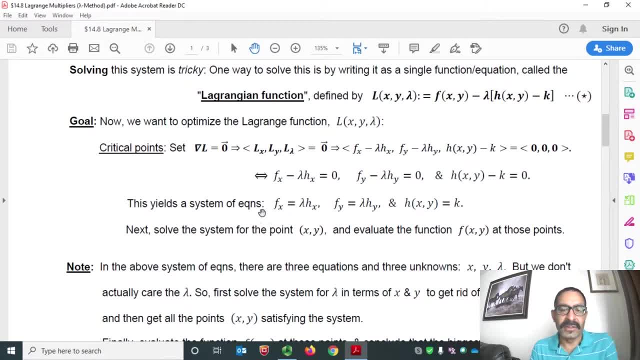 equations here. So we do have this system equation here: f x equals to lambda h x. f y equals to lambda h- y. So next solve the system for the point and evaluate the functions at those points. Quick note about this idea here. 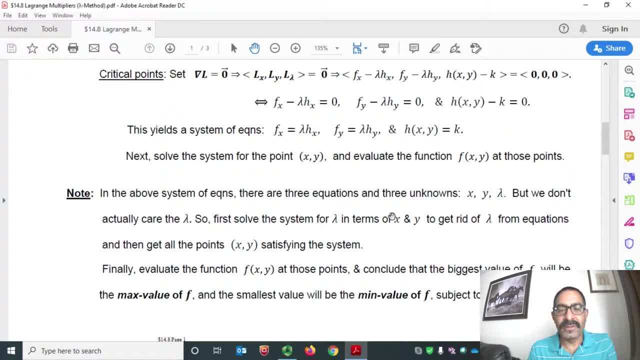 In the above system of equations there are three equations and three unknowns. Here we have one equation, two equations, three equations and we have unknowns are x, y and lambda. But we don't actually care the lambda. So first solve the systems for lambda in terms of x and y to get rid of lambda from the equations. 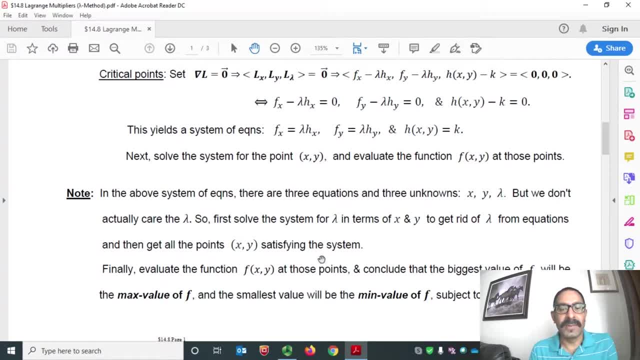 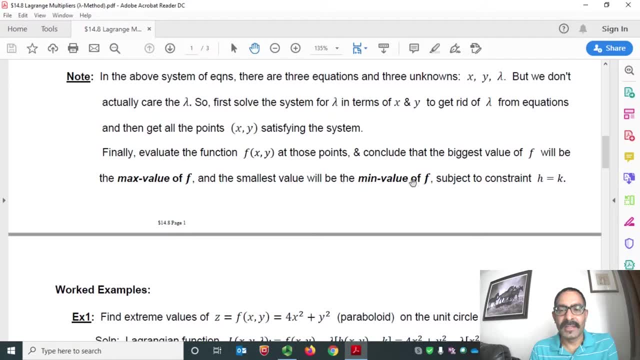 and then get all the points, x, y satisfying the system. Finally evaluate the functions at those points and conclude that the biggest value of f will be the maximum value of f and the smallest value will be the minimum of f, subject to given constant. So that's it. 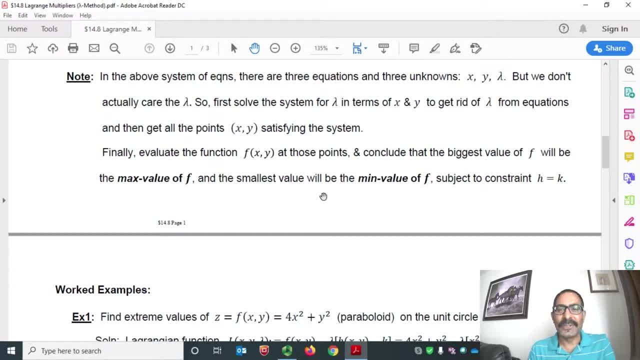 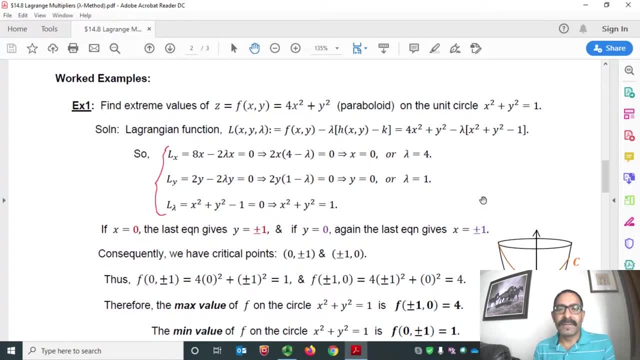 With this idea. now let's do some example. Let's move on. Example one: find the extreme values of the surface. here, f equals 4x squared plus y squared. It's a parabola, by the way, On the unit circle, where x and y satisfy this equation, x squared plus y squared equals: 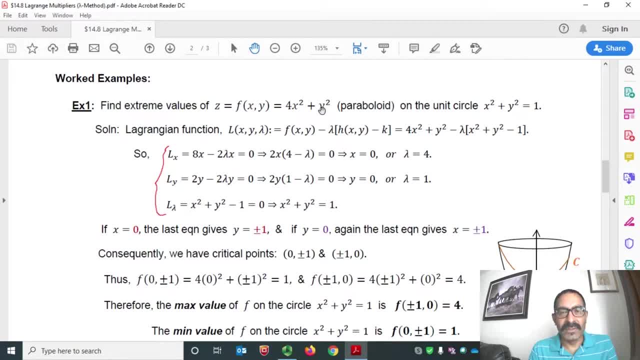 to 1.. So here this is our f of x, y And this is our h of y. This is x, y, which is k, k is 1 here. So let's begin the solutions. Define the Lagrangian functions L, x, y. lambda equals to objective functions minus lambda. 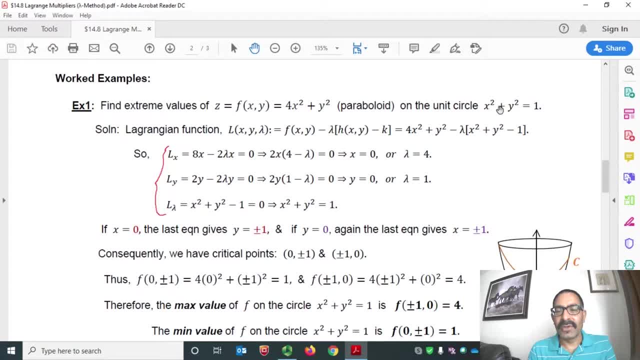 times the constraint here: x squared plus y squared minus 1, and this is the f x y And this is the lambda. So next let's find the critical point, Find this, The partial derivatives. Find L x. L x equals to here's 8x minus 2, lambda x. 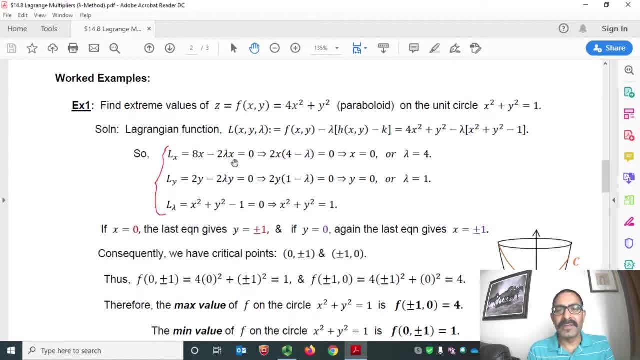 Keep in mind that we are taking partial derivative with respect to x, So y's are constant, Set equals to 0.. Simplify It gives us here's: either x equals to 0, or lambda equals to 4.. By the way, we don't care the lambda value. 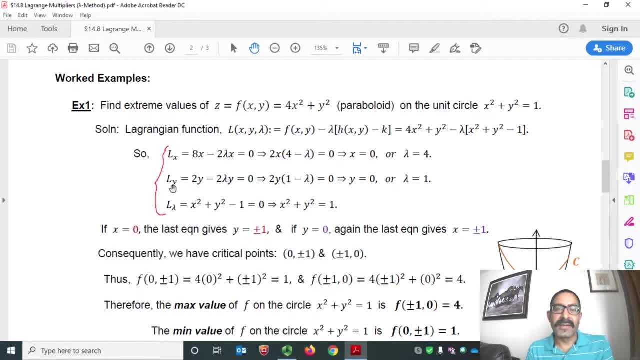 We only care. x equals to 0.. The second line here: escape Yamada. for x squared equals 1.. The third line here: here including √hHOx, H is the value of lambda squared plus a joint square. 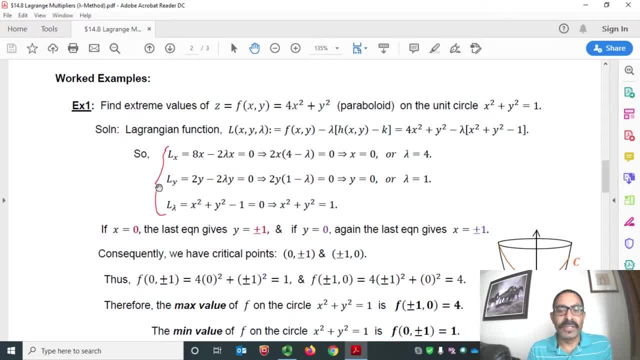 The variable for the void function, here the 0 state. these espaço value is 0.. So dou NOT equal to and s squared of x squared equals 1, or less than do is equal to ¼ of 1.. the partial derivative l with respect to y is 2y minus x square 0, 2 lambda y. so minus 2 lambda y. 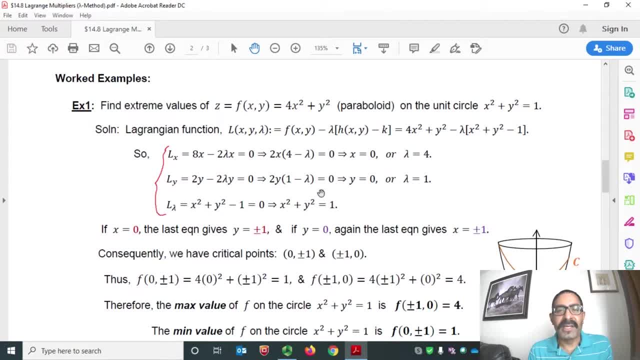 set equals to 0. simplify it gives us y equals to 0 or lambda equals to 1. again, we don't care. lambda value. third line: here take the partial derivative l with respect to lambda. so that means x square terms 0, y square terms 0, so only here. so that means x square plus y square minus 1. 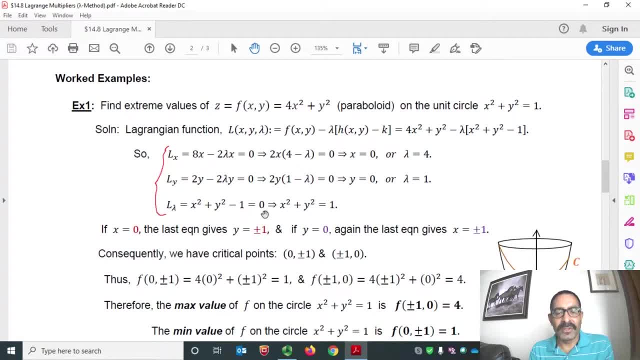 x square plus y square minus 1 set equals to 0. i mean here i forgot the minus sign. i have to multiply by minus, but when you are setting equals to 0, that minus disappears. so we have x square plus y square minus 1 equals to 0. this implies x square plus y square equals to. 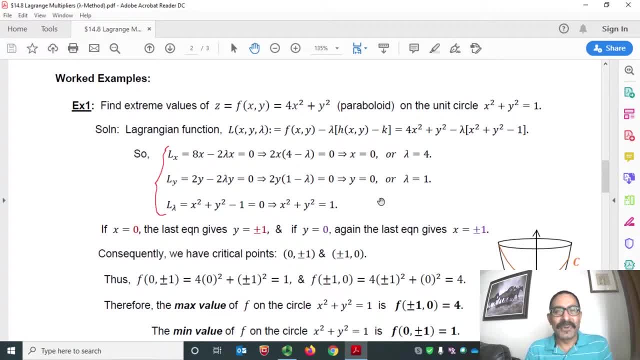 1. i hope this you make sense to you all. so the next. so let's find the value of fraction. y means: put x equals 0 in this equations. put y equals 0 in this equations. so if x equals 0, the last equation gives y equals. 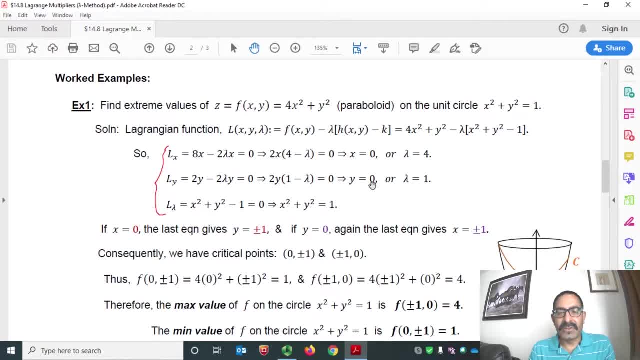 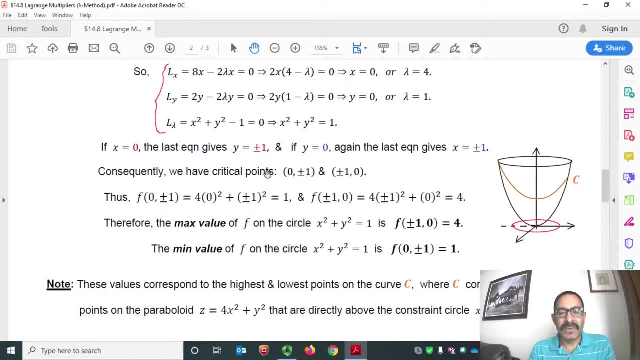 to plus minus 1. and if y equals to 0, again the last equation gives x equals to plus minus 1. so we have the critical point: when x is 0, y is plus minus 1. when y is 0, x is plus minus 1. 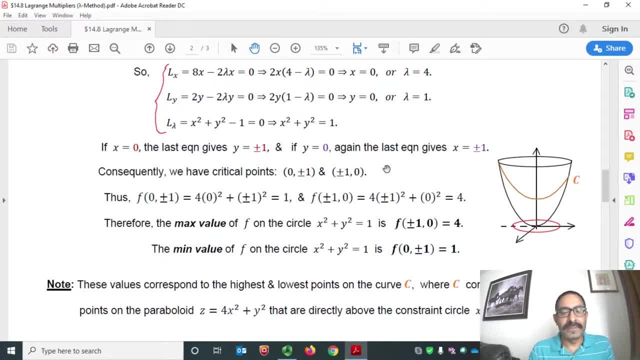 minus 1.. So we have 4 critical points. Next let us evaluate the functions at those critical points. So here: f at 0 plus minus 1 gives us, it is our function. here: f, x square plus y square. 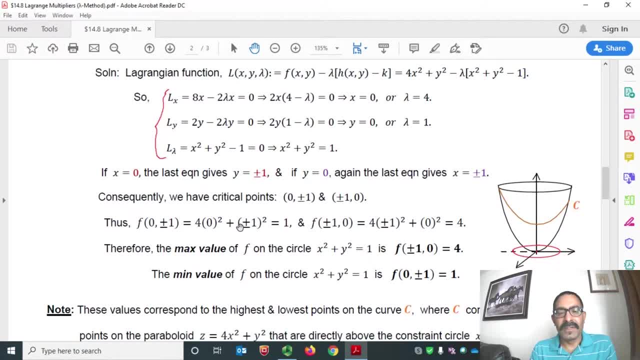 So 4,. this is the x value, this is the y value. Simplify gives us 1.. Similarly, evaluate the f at this critical point, which gives us 4.. So that means we found the maximum is 4,. minimum is 1,. 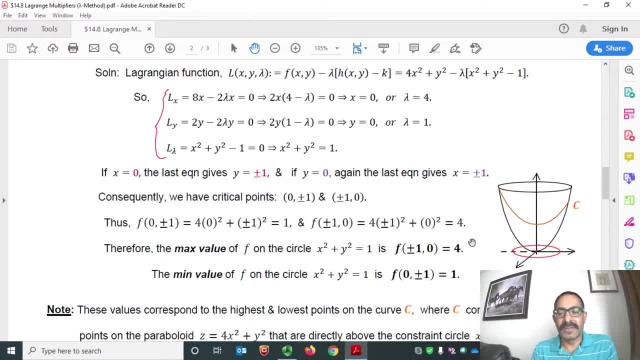 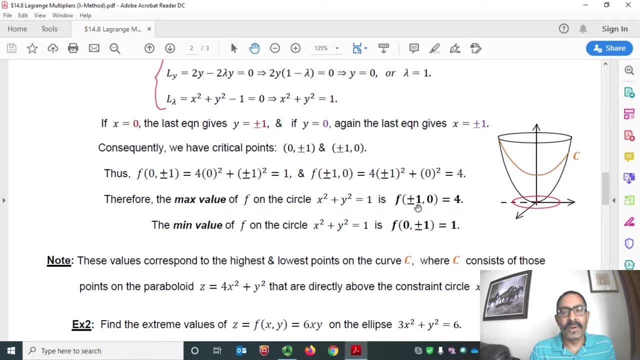 maximum at these two points, minimum at these two points. So the maximum of f on the circle is 4 at this point plus minus 1, 0, and minimum is 1 at this point, 0 plus minus 1.. I hope this computation makes sense to you all. 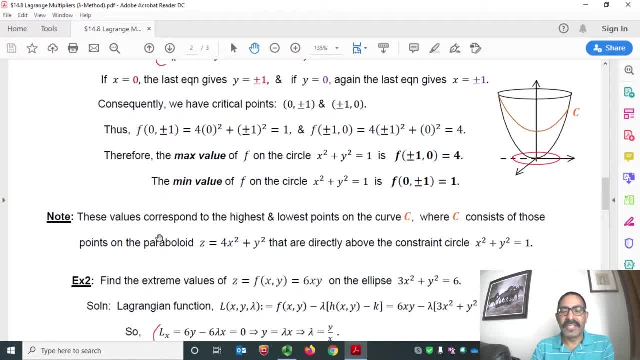 So actually these values correspond to the highest and lowest point on the curve, where the curve consists of those points on the paraboloid that are directly above the constrained circle. So on this curve, which is just above this constrained circle, 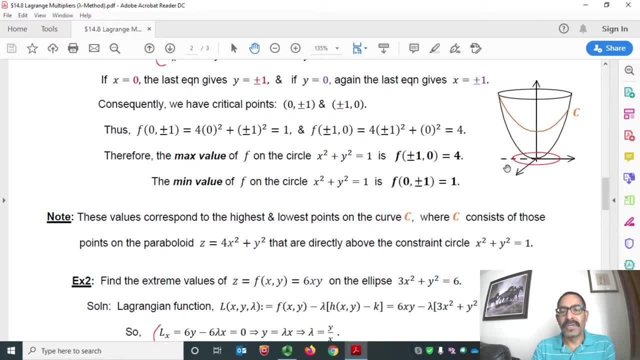 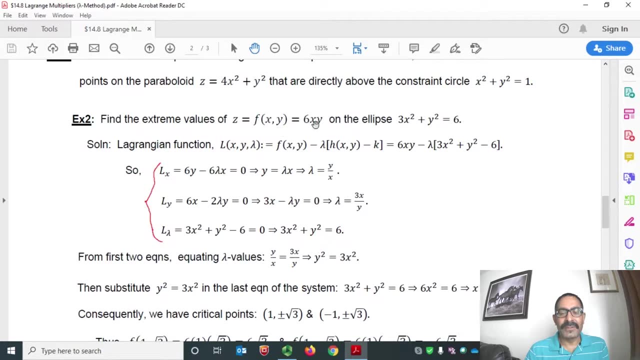 we have. the highest point is 4 and the lowest point is 1.. Great, I hope this idea makes sense to you all. Now let us move on Example 2,. find the extreme value of functions f equals to 6xy. The constrained curve is the. 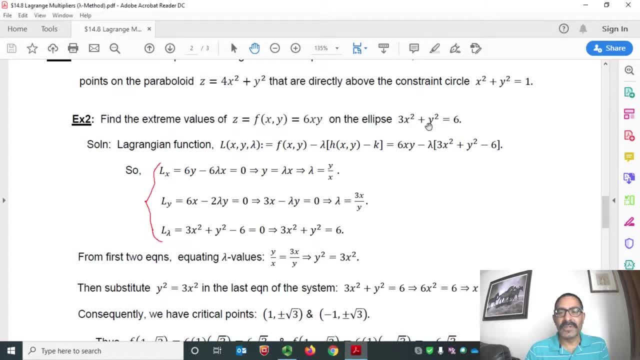 ellipse 3x square plus y square equals to 6.. Begin the solutions. This is the routine computation. So let us define the Lagrangian functions: L equals to objective functions minus lambda times the constraint which is here: 6xy minus lambda times 3x. 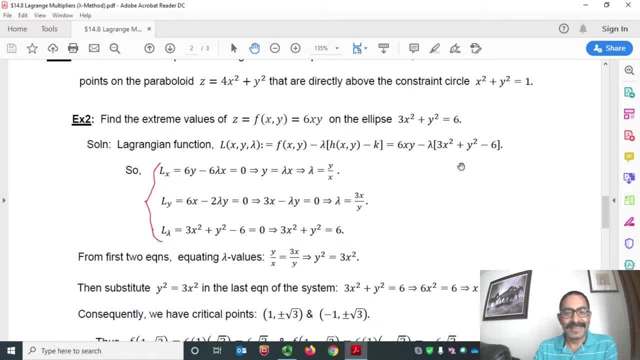 5y plus 2y. squared plus 3x- Y squared plus 3x, The function f equals to the masked function. This is the 청- convected function. the constant function f is nothing but an element, and when you multiply that over the given element, 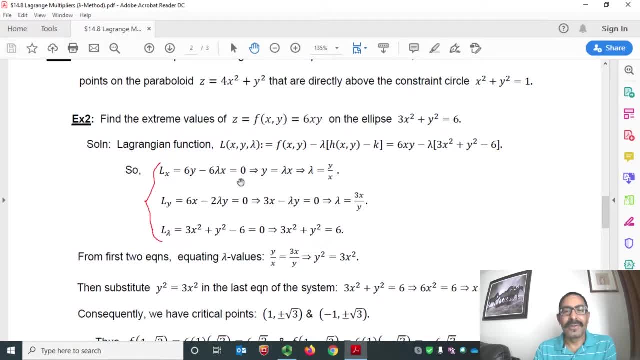 you get that f equals to f 4 times f plus f and you get f prime f plus f prime, and f prime f is nothing but f 4, and f prime f is nothing but f prime x. So if f is not, equal to f. the function f equals to f 2, what we have here is f prime x times f2, which makes 6y plus y square, minus 6y over x. That means f square is equal to f x squared, which. 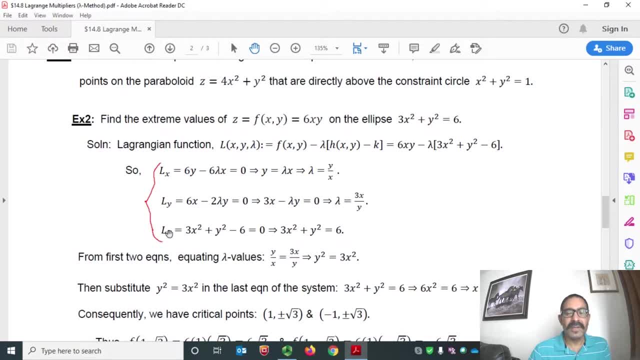 is x squared minus y squared again, is equal to x squared, which means z squared. Now, I hope, x over y. similarly, l lambda equals to 0, gives us 3 x square plus y square equals to 6, by the way, always the partial derivative of Lagrangian functions with respect to lambda, when we set 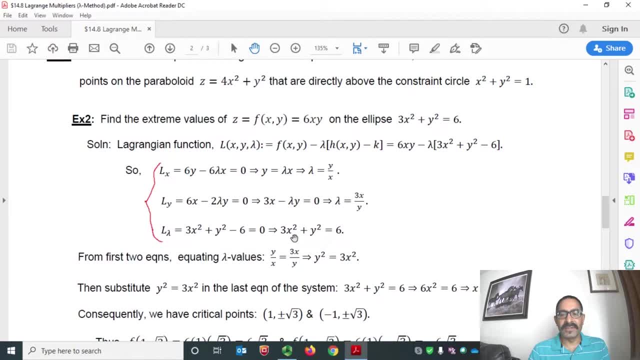 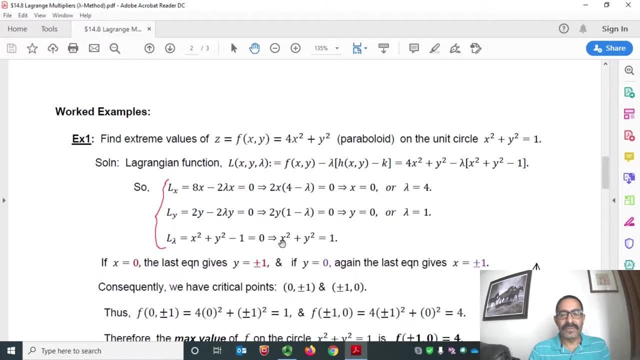 it equals to 0. it gives us always the constraint curve. so this is the constraint curve: 3 x square plus y square equals to 6. is here: 3 x square plus y square equals to 6. in the earlier case, also the same l lambda equals to 0. gives us x square plus y square equals to 1, which is here. that's the idea. 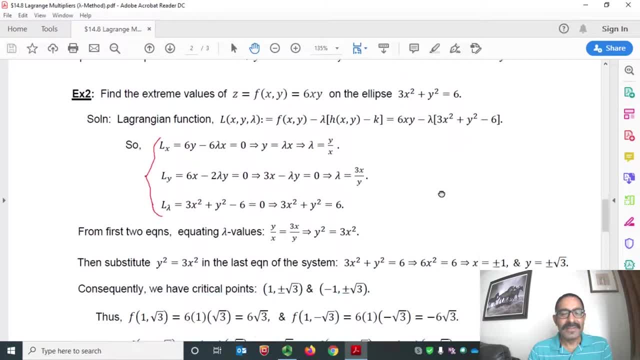 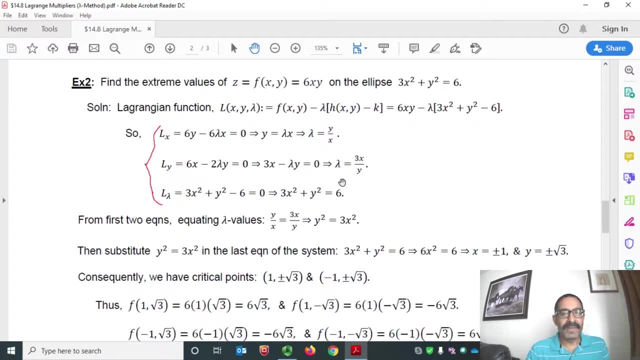 great, so let's move on. so then, now our goal is to find the value of x and y. again, we don't care, the lambda value. so from first 2 equations the same lambda, let's equate these two lambdas. that means equate the right hand side. so 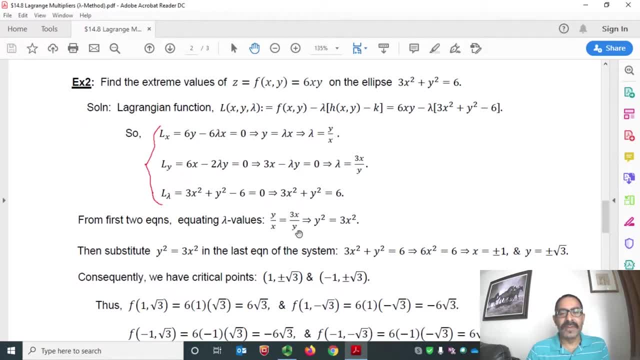 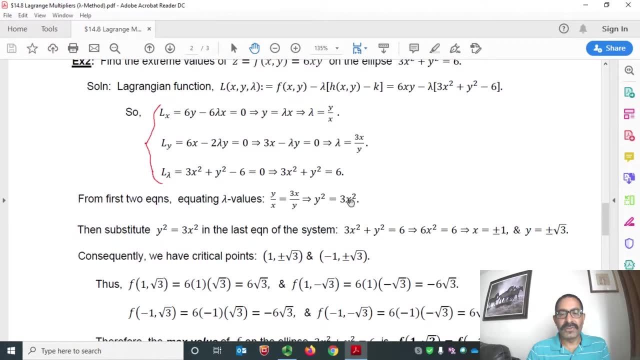 y over x equals to 3 x over y. then from here y square equals to 3 x square. and then substitute: y square equals 3 x square. in the third equations 3 x square plus y square equals to 6 becomes 3 x square and y square is again 3 x square. so total 6 x square equals to 6. solve for x. 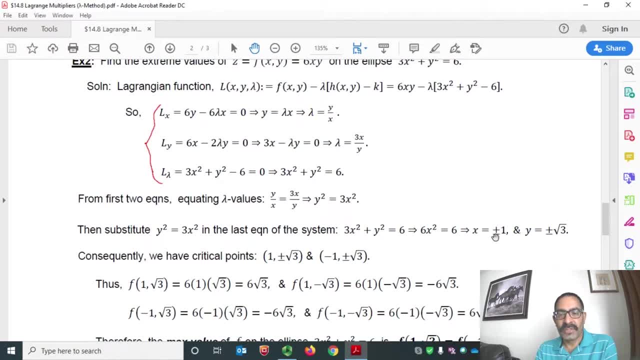 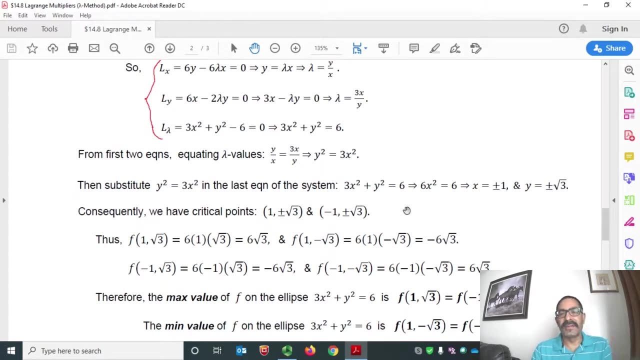 x equals to plus minus 1. put y equals to plus minus 1 back on y square equals 3 x square. then y equals to plus minus radical 3. so consequently we have critical point 1 plus minus radical 3 and minus 1 plus minus radical 3. again for critical point to next step, evaluate our function at those point. so here's F at 1, radical 3. again, our function is 6 x 1. next step: eliminate our function at those. plug here. F at 1, radical 3, again. our function is 6, x, all over x, 3, knowsります one radical three, which one. 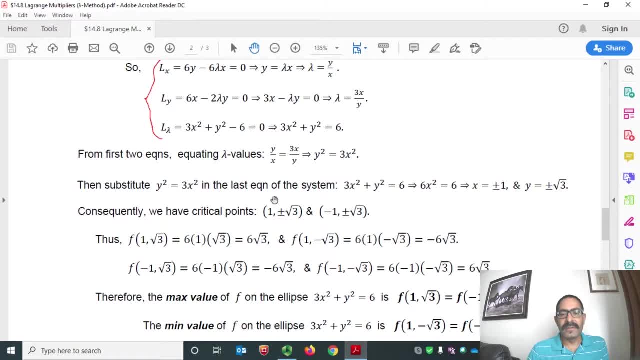 yes, if you are in the home system. next, with the remember this play value plus, or to capacitor F has no error at one. radical three unstable appears here, so we will see how that will make you know. so that, anyway, our function, this function, this is it we are and we concentrated. 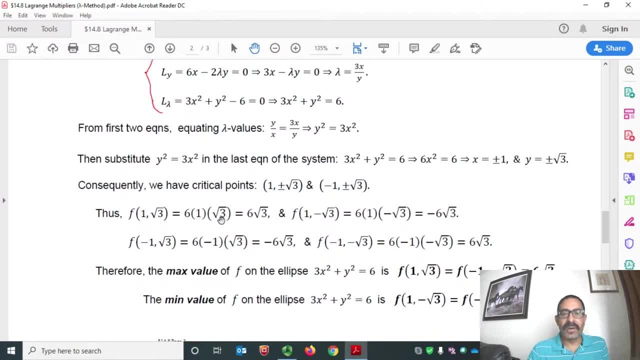 blue orange theme in theorer, social terms here, so that all in the other expression plus simple: and x, y, 6, x value is 1, y is radical 3, it turns out that 6 radical 3,, similarly f at. 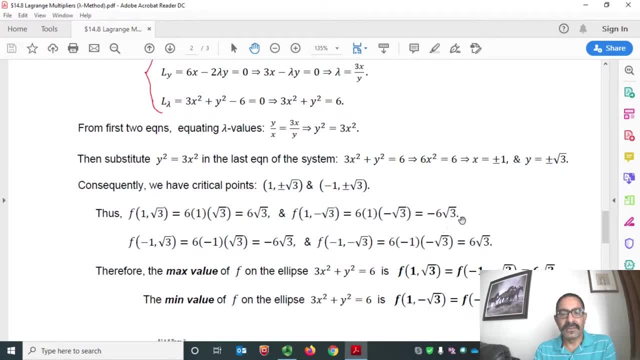 1 minus radical 3 turns out to be minus 6 radical 3,. similarly, f at minus 1 comma- radical 3 turns out to be minus 6 radical 3,. and f at minus 1 comma- minus radical 3 turns out. 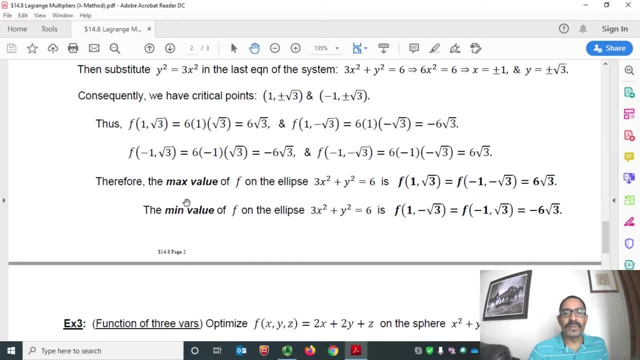 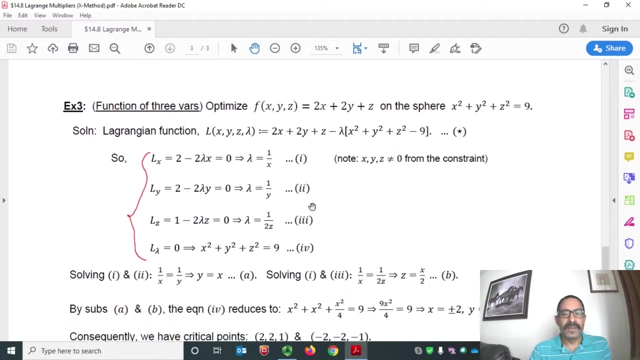 to be 6 radical 3.. Therefore, the maximum of f on the ellipse is 6 radical 3 at this 2 point and minimum is minus 6 radical 3 at this 2 point. I hope this makes sense to you all. Great, let's move on. Let's do for function of 3 variables. Example 3, optimize. 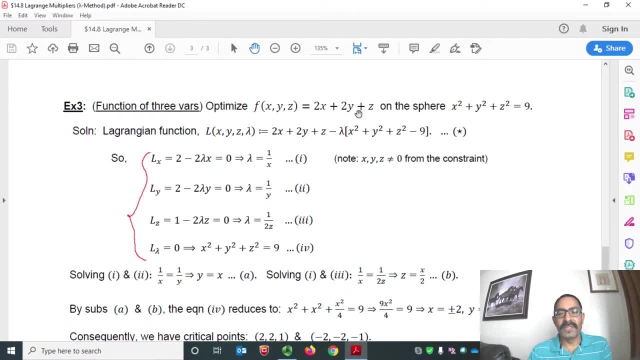 the function of 3 variables, which is 2x plus 2y plus z, And on the sphere x square plus y square plus z square, equals 9.. By the way, this is also a level surface. So let's begin the solutions. Define the Lagrangian functions. L equals. 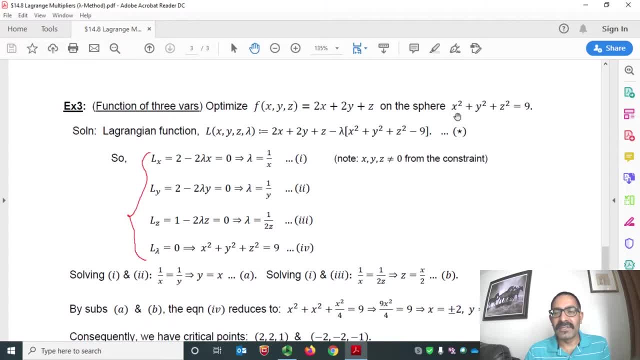 to objective functions minus lambda times this constraint. Then take this bunch of partial derivatives here, Lx set equals to 0, and this gives lambda equals to 1 over x equation 1.. Similarly, partial derivative of L with respect to y set equals to 0, gives us equations: 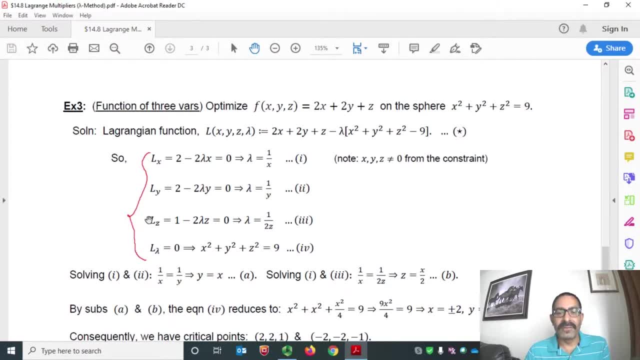 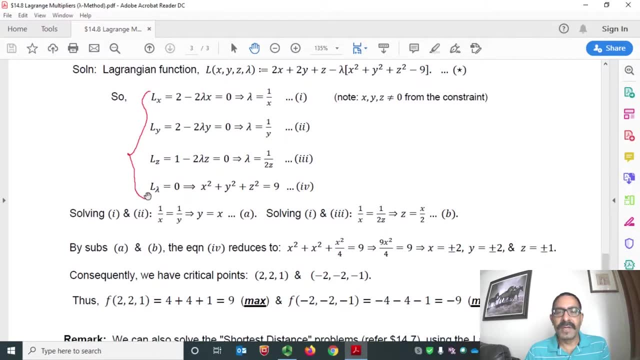 2. Similarly, partial derivative of L with respect to z, set equals to 0, gives us equation 3.. Similarly, partial derivative of L with respect to lambda, set equals to 0, gives you this constraint curve equation 4.. So now our goal is to solve these system equations. 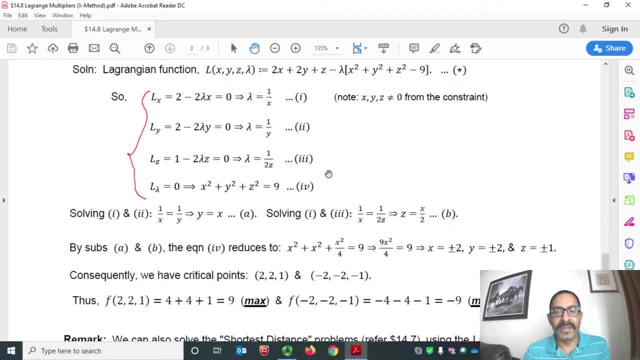 And find the value of x, y and z. Again, we don't care, the lambda value Solving first and second. same lambda equate: 1 over x equals to 1 over y. This implies y equals to x equation. 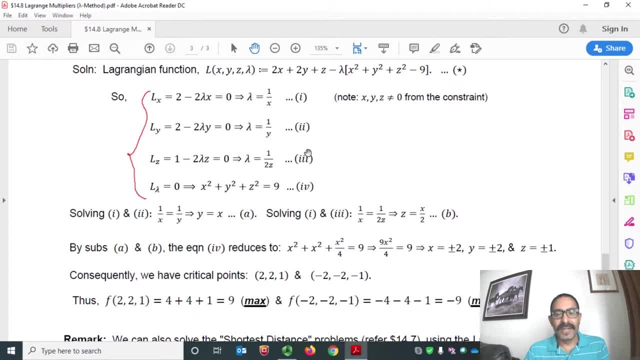 a Solving first and third again, same lambda equate: 1 over x equals to 1 over 2z. This gives z equals to x over 2, equation b. Then substitute the values for the first and second and find the value of x, y and z. 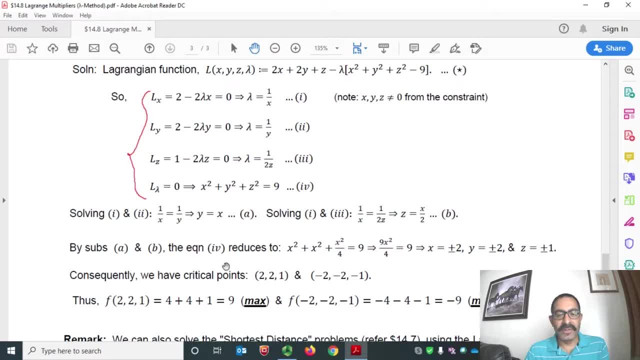 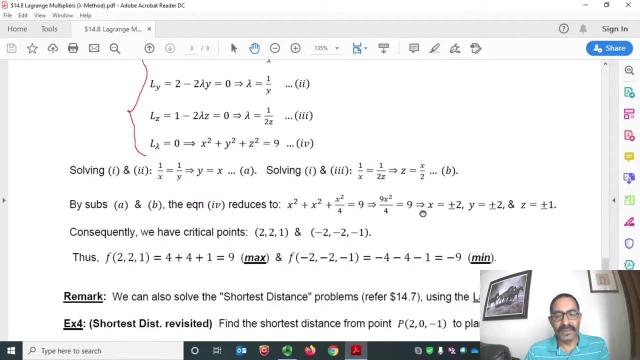 Now, when you put the values of equation a and b into equation iv, then equation iv reduces to: x squared plus y is x. So again, x is squared plus z. z is x over 2 squared equals to 9.. Solve for x. This gives us x equals to plus minus 2.. Since y equals to 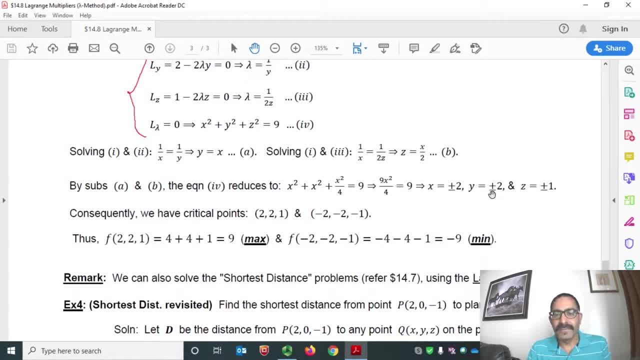 x, so y is also plus minus 2.. Then z equals to x over 2, equation 3. Again, y equals 2.. z equals x over 2,, so z equals 2 plus minus 1.. So we found the critical point. 2 comma. 2 comma 1. 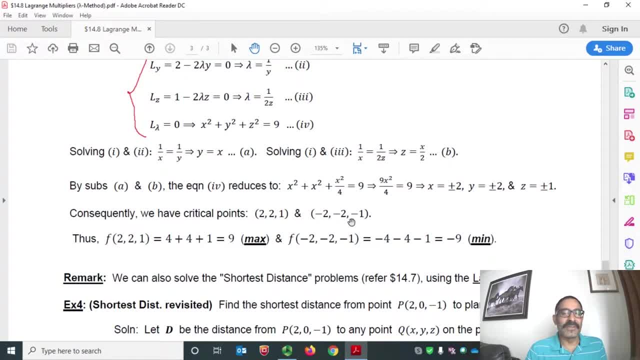 and minus 2 minus 2 minus 1, two critical point. The next step: evaluate the functions at those critical point. We found here: f at 2 comma, 2 comma 1 is 9 maximum and f at minus 2 comma minus 2. 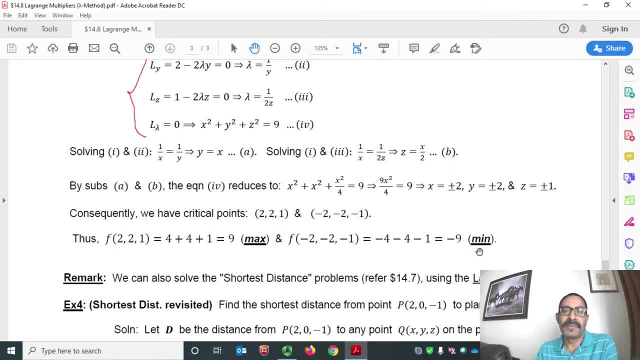 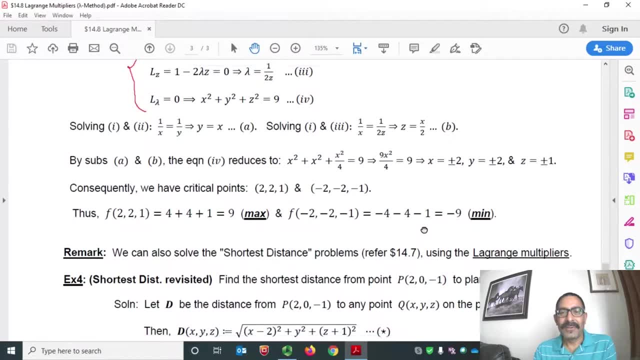 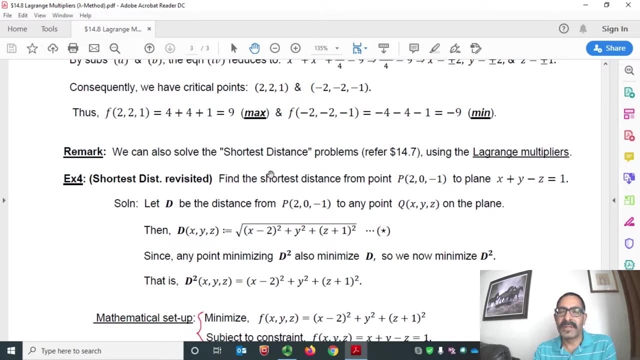 comma minus 1 is minus 9, a minimum. I hope this answer makes sense to you all. Quick remark: we can also solve the shortest distance types problems. We did these types of problem in section 14.7, but this time using Lagrange multipliers means using lambda. 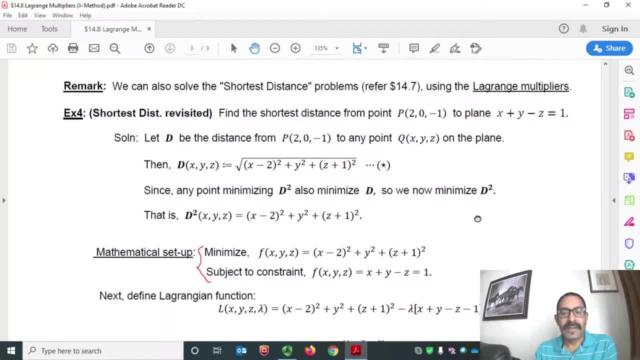 Let's do the example 4.. Let's revisit the shortest distance problem that we did in section 14.7.. So the question was: find the shortest distance from the point P to the plane. The plane is: x plus y minus z equals to 1.. 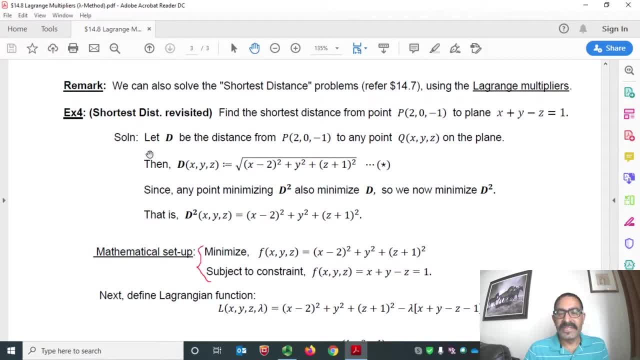 So begin the solutions. So let d be the distance from given point P to any arbitrary point Q on the plane. Then our d equals to this equation star. This is just the distance formula, Since any point minimizing d square also minimizes d. 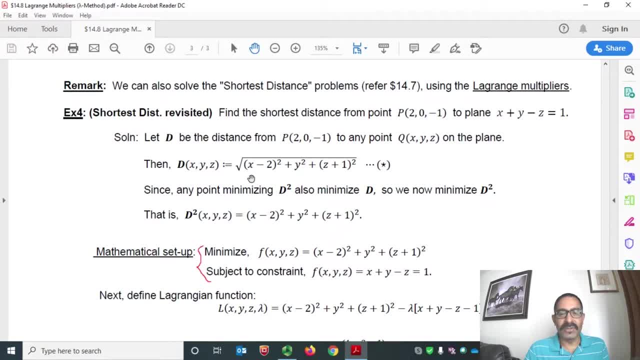 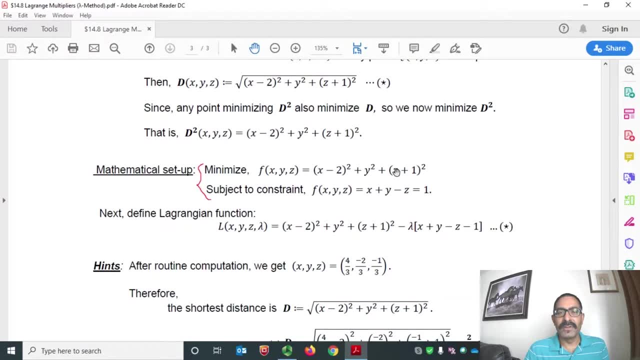 So we now minimize d square, So d square equals. to just get rid of this radical, we have these equations. So the mathematical setup for Lagrange's method is: we are minimizing because we are finding the shortest distance, So we want to minimize, So minimize the functions f. 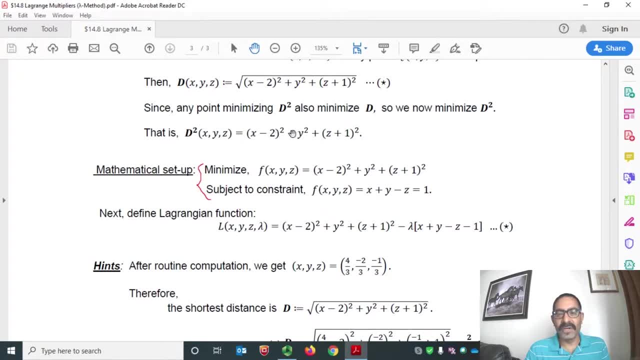 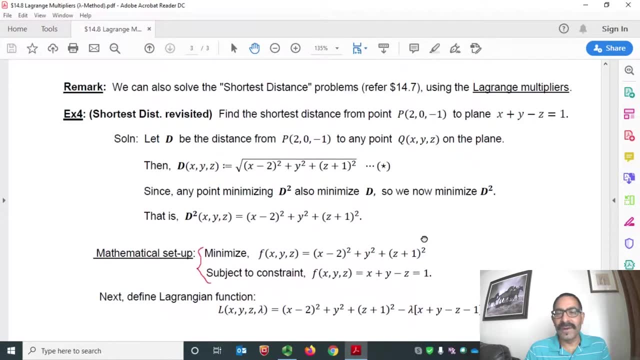 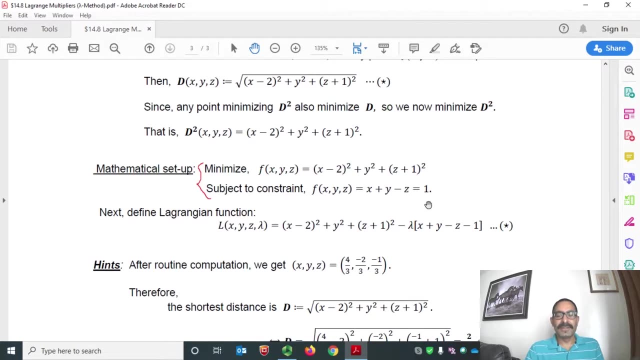 which is d square. that means x minus 2 outside square plus y square plus z plus 1 outside square. subject to constraint, those x, y, z should satisfy this equation of plane. x plus y minus z equals to 1. then just follow the routine computations means define the lagrangian functions, so lagrangian.